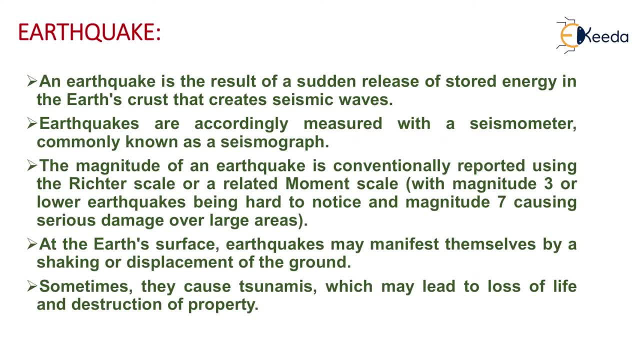 accordingly measured with a seismometer commonly known as a seismograph. The magnitude of an earthquake is conventionally reported using the Richter scale or a related moment scale, with magnitude 3 or lower earthquakes being hard to measure At the earth's surface. earthquakes may manifest themselves by a shaking or displacement of the 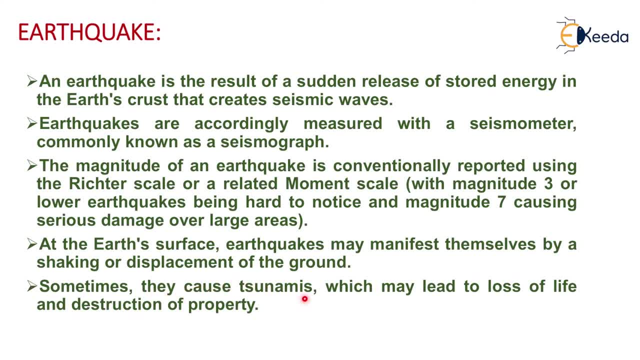 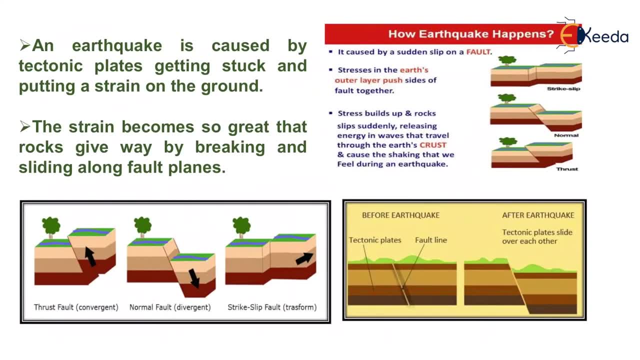 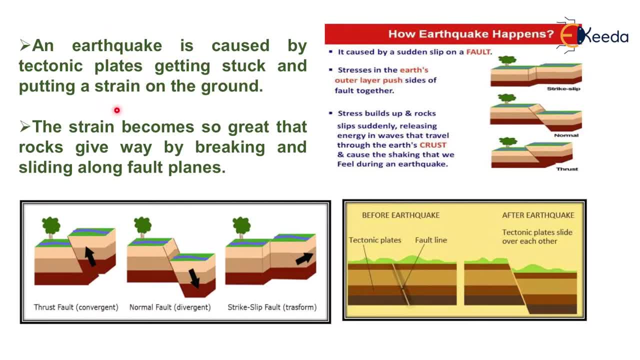 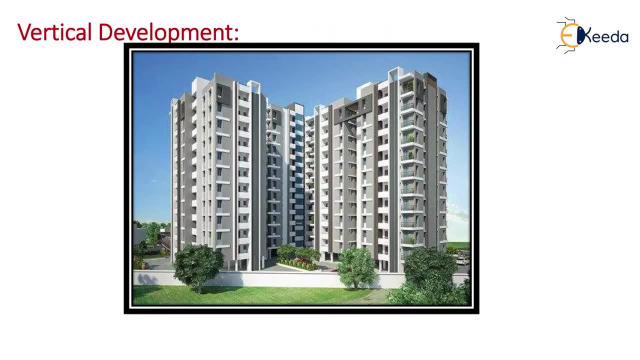 baits getting stuck and putting a string on the ground. thus strain becomes so great that rocks gives weight by breaking and sliding along false-plane. Now, what is vertical development and what is horizontal development? Due to current scenario, there is rapid growth in population and it is easy to imagine these loops, shifts and Tellar stretches in fixtures. princes, canon, The gesprochen fusionventure calms the human mind to the SAMR. 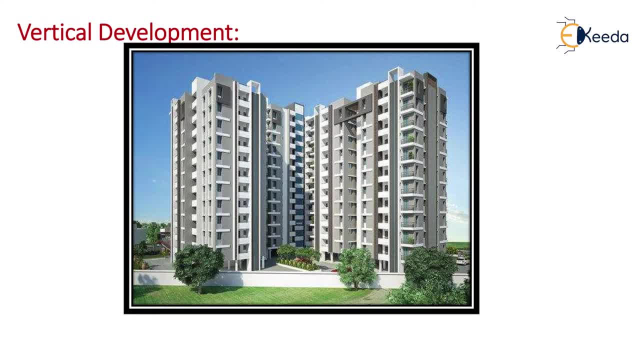 land area requirement is also increasing as well as cost area increasing. As we know, there is limited space on earth surface for residential building, offices, shops, etc. In metro, city, mega cities, most of the structure are high building since population density more and as increasing at high rate. So we are moving toward the vertical development. 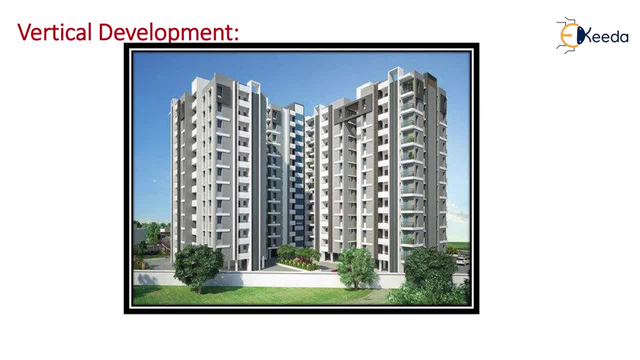 in which we are constructing multi-storied building for residential as well as for offices. Therefore, vertical development means to sustain greater population at one place, and there are the development done in vertical direction. There are many advantages and disadvantages of vertical development. One important disadvantage is earthquake damage. 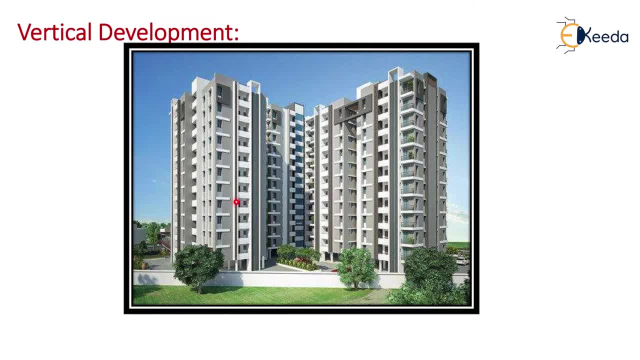 and if the height of building is increasing, then damage due to earthquake also increases. To decrease or for minimum damage, we should strengthen our structure by designing structure for earthquake resistant design. For this, first, it is important to know that the intensity or magnitude of earthquake arises in that area, city or state. 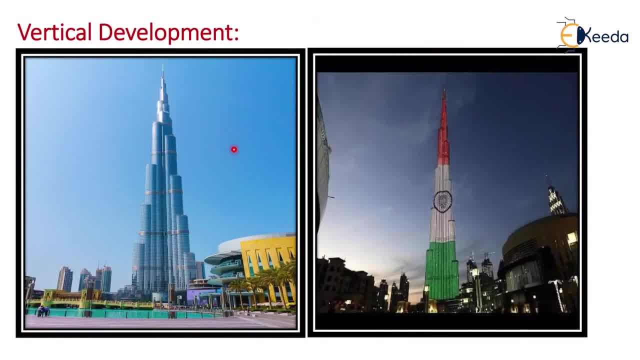 Now, taking an example of Burj Khalifa. it is one of the tallest structure in the world. It is proposed to design the structure for earthquake intensity of 5.9 magnitude from their recommended codes, But it is designed for an earthquake intensity of 7 as per the consideration of worst condition. 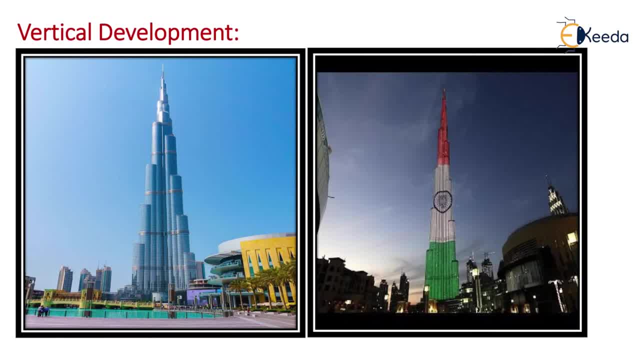 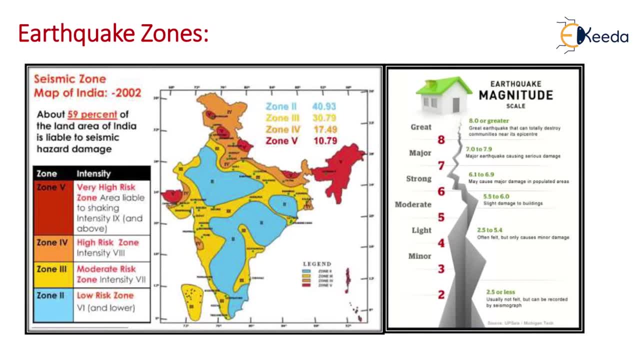 Therefore, heavy protection is given against earthquake. Now we will see what are the provisions. criteria or fulfillment are considered for design of earthquake resistant building and where it is given. It is given in Indian Standard Code IS 1893-2002. As per Indian Standard Code, in India earthquake is divided in 5 zones. 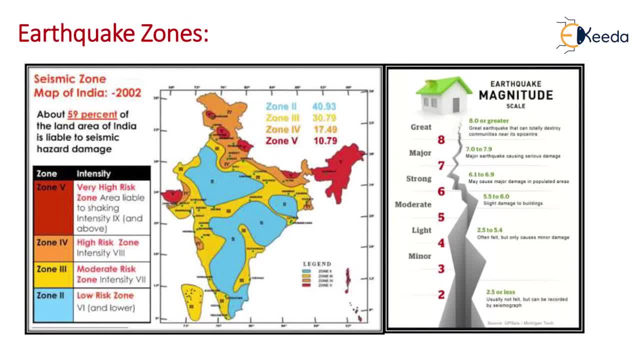 But now 1st and 2nd zones are merged. Therefore 4 zones are there. These zones are divided state wise. This is the map You can see. from this you will understand how zones are divided In different state and this map also shows different zone consist of range of magnitude of earthquake. 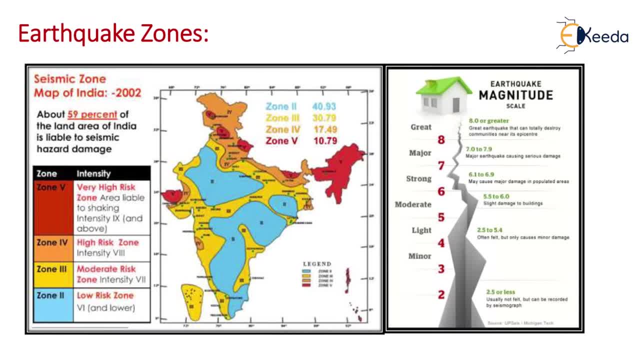 It is important to keep in mind that the design of earthquake resistant building, the design consideration, are not limited to the calculation of live load, dead load, earthquake load, wind load and then total load. After this distribute overall load And design is finished. 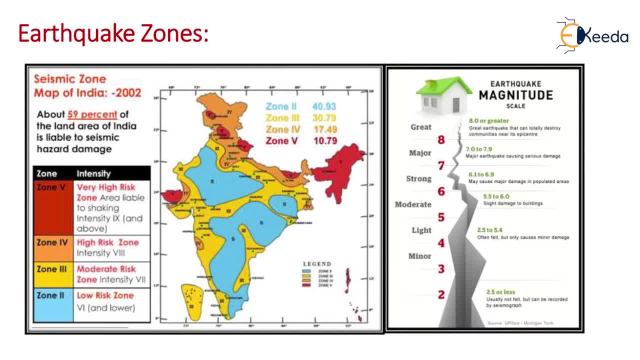 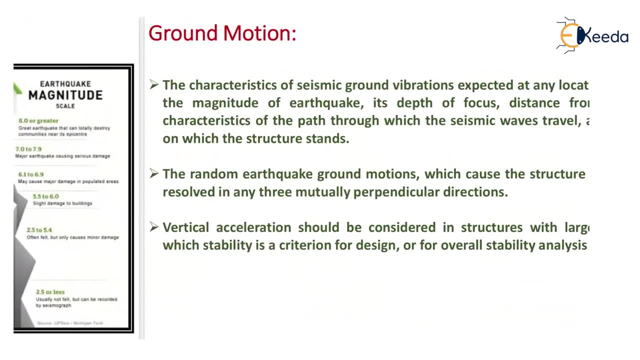 And provide some provisions. No, this is not. We have to also apply some concept like shear wall design, detailed ductility, strong column and weak beam concept, floating beam concept. Now moving toward ground motion. The characteristic of seismic ground vibrations expected at any location depends on the location of the earthquake. 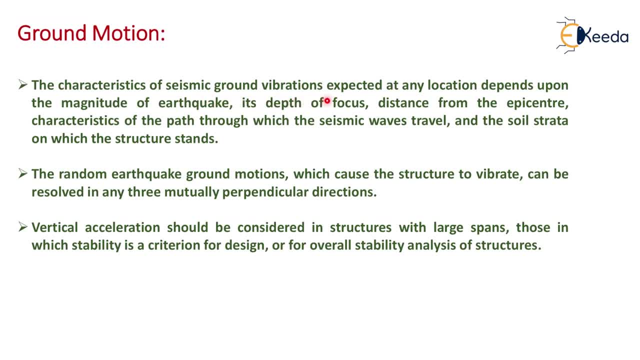 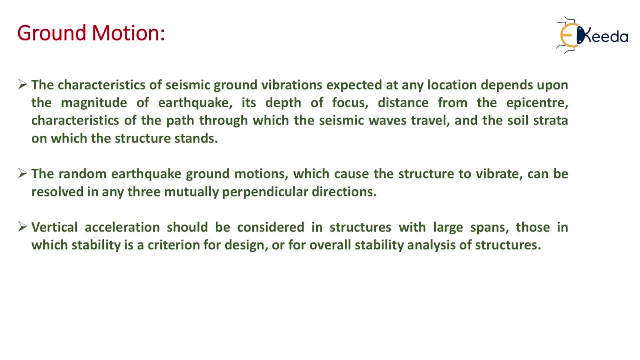 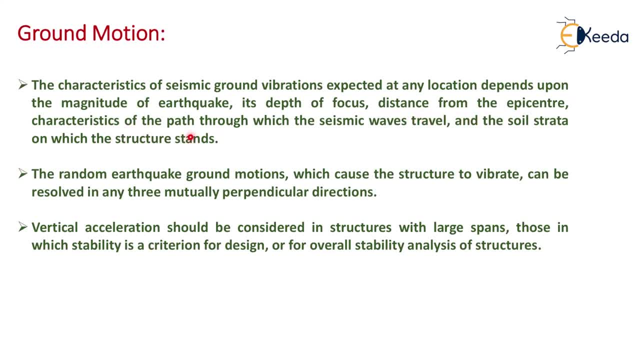 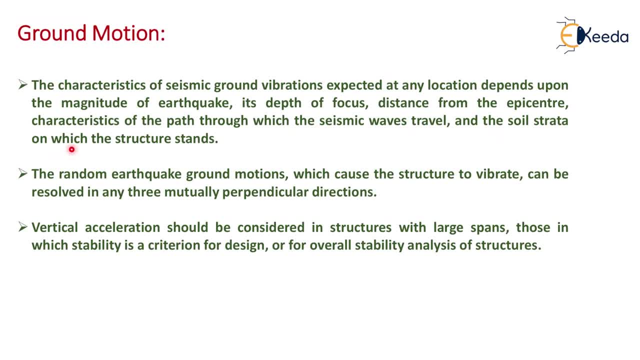 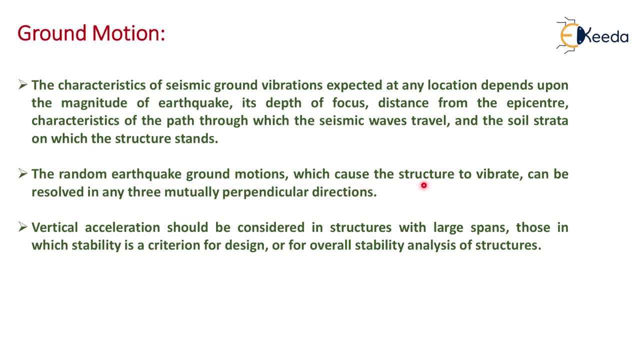 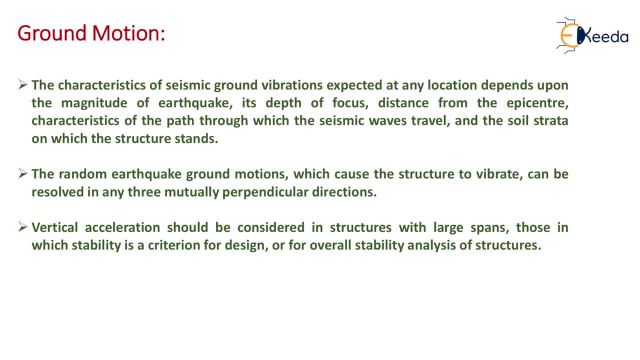 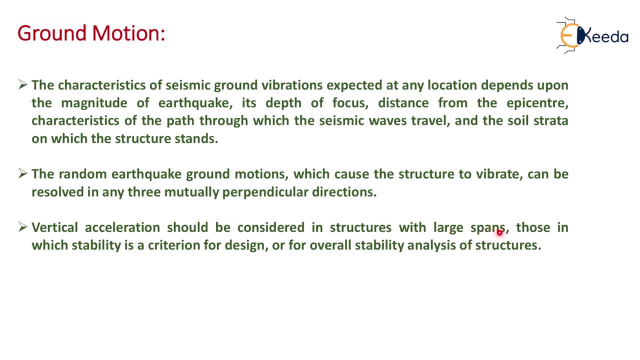 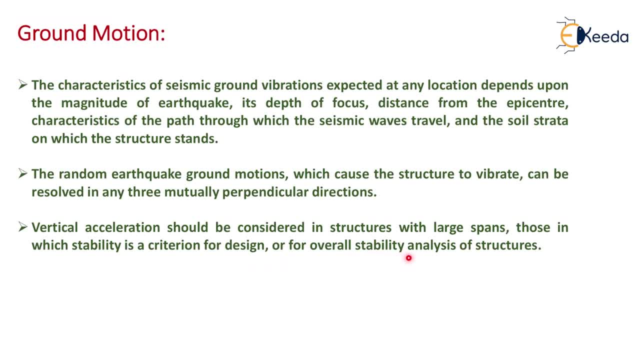 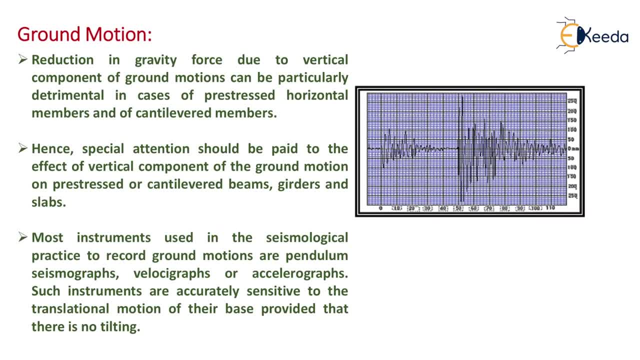 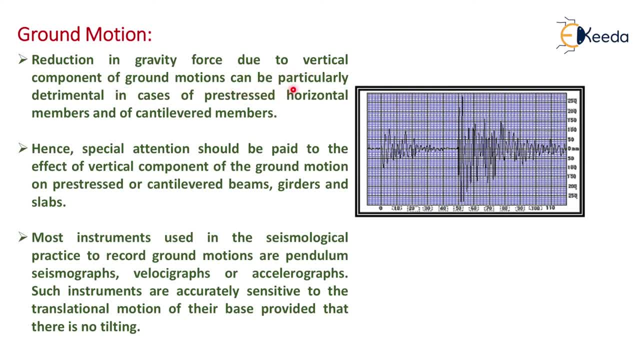 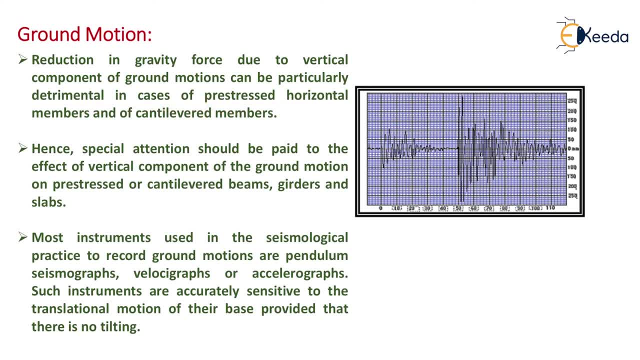 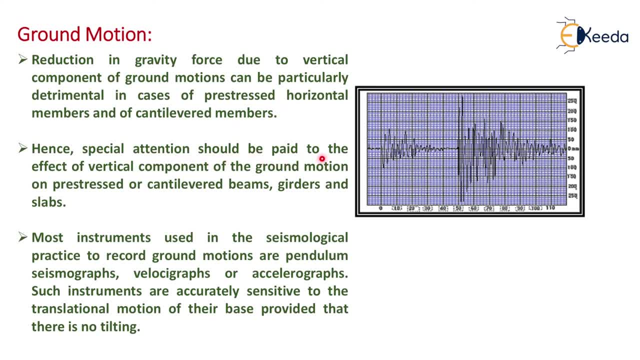 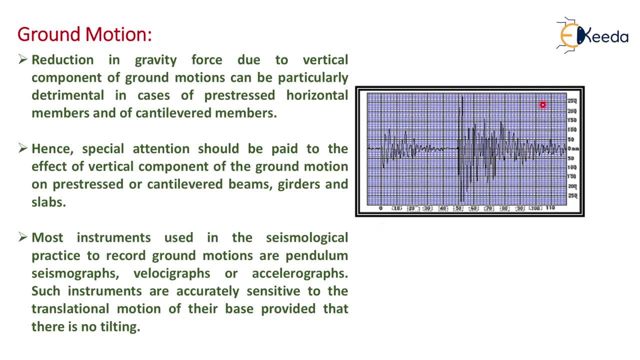 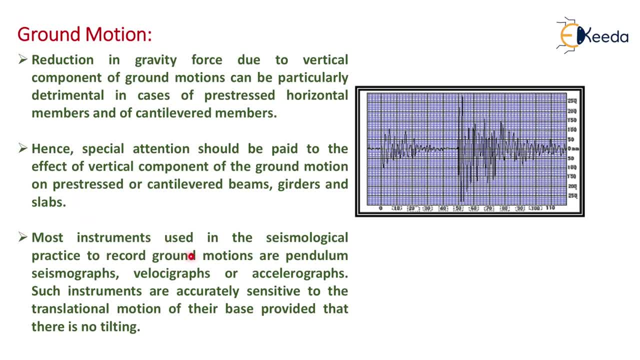 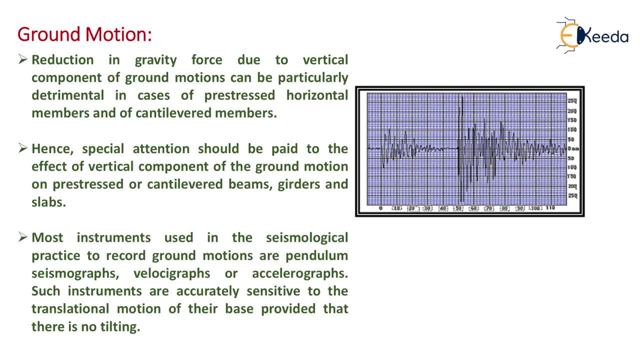 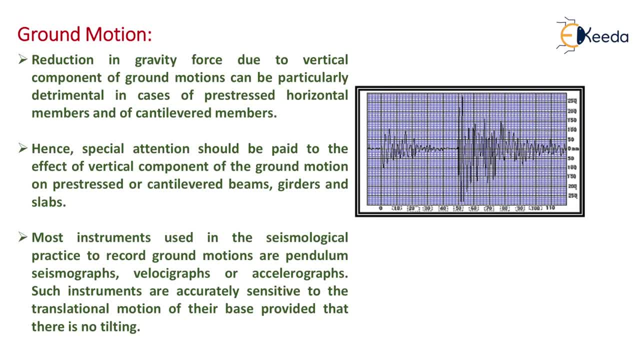 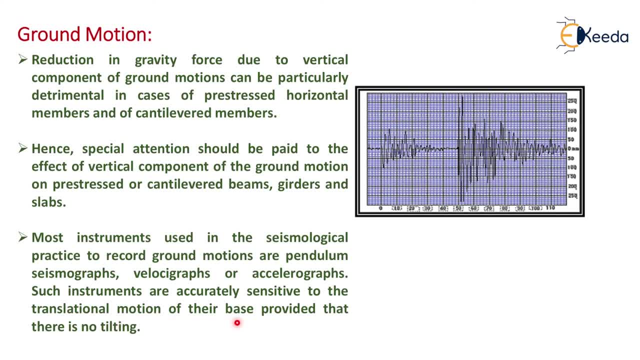